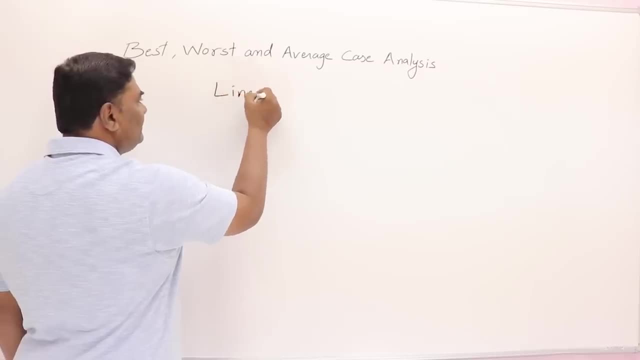 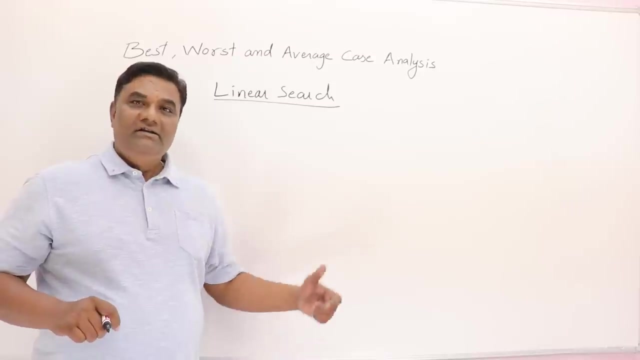 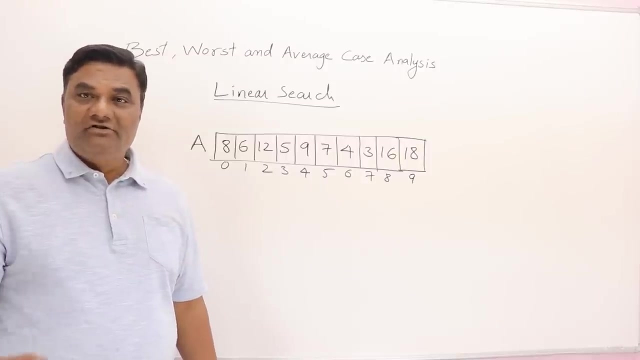 The first one is linear search, Linear search. Linear search: If a set of elements, list of elements, are given, then when we are searching for any element in that list, then we have different search methods available, like linear search, Linear search and binary search. Let us see how linear search works Here. I have a list of 10 elements and in this I want to search for some key element. Let us say I want to search for key element 7.. 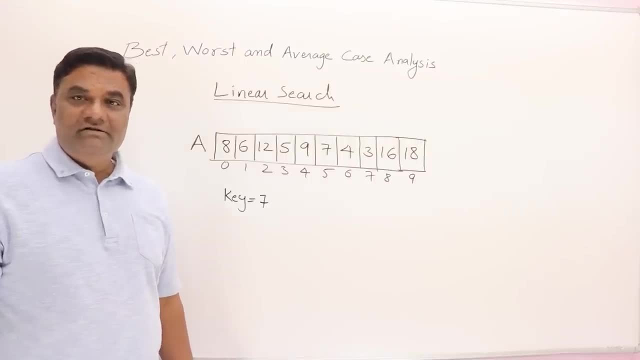 What is the method for searching for a key element? For looking for a key element, the linear search will start scanning the list from left hand side by checking each element at a time. So it will start checking whether this is 7.. No, Go to the next element. Is it 7?? No, Is it 7?? Is it 7?? So it will go on checking all the elements until either it finds an element- Yes, the element is found. 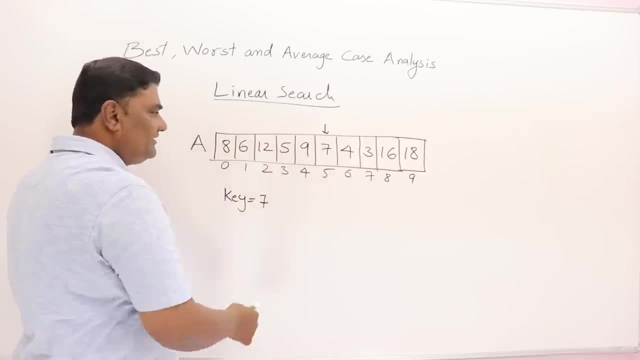 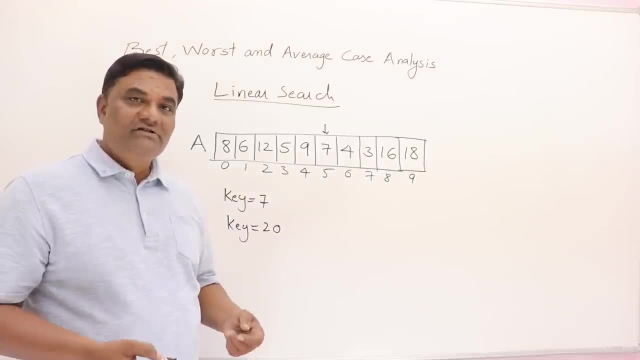 So when we search in a list, the search may be either successful or it may be unsuccessful. So for 7, it was successful and we found it at index 5. And 20 is not found when we have checked the entire list. 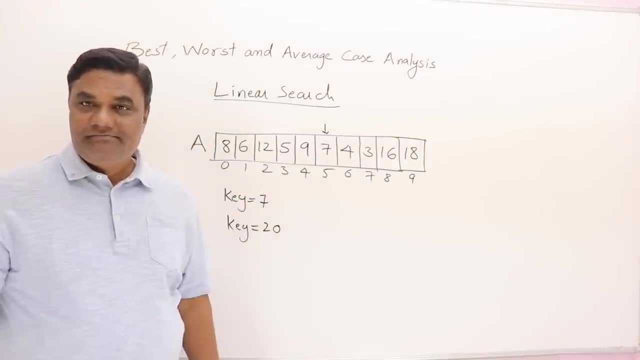 So this is how linear search works. Now let us understand what is best case and what is best case time. What is worst case, What is worst case time? We will find out in this linear search in Gotham. First, let us see what is best case. 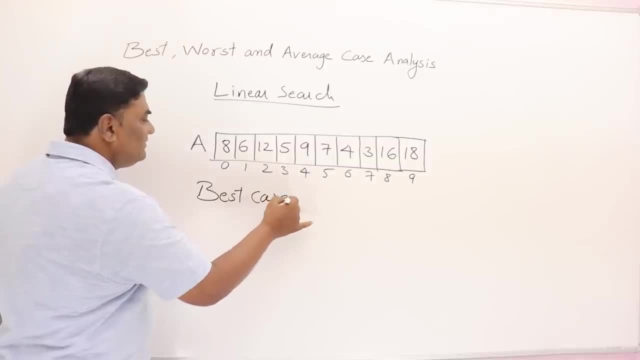 Best case In case. if you are searching for a key element which is present at first index, then it is best case In case the case you may be searching for any element from the list, but if you are searching for a key element which is present at index first index, the very beginning index, then that is best case. 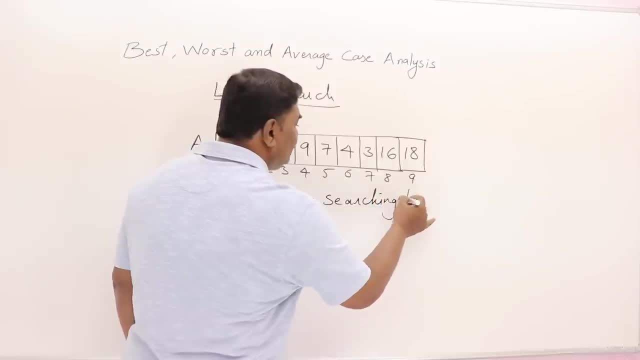 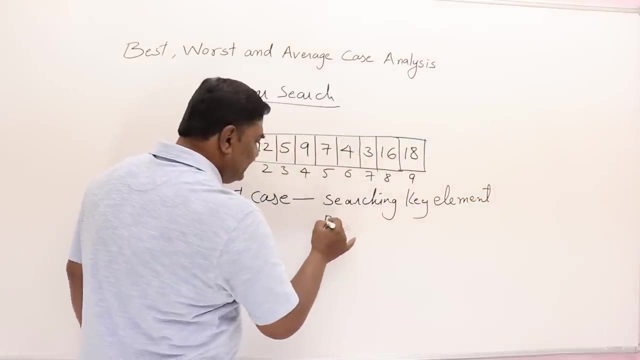 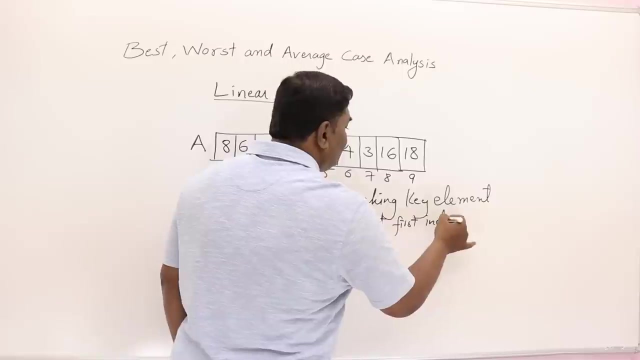 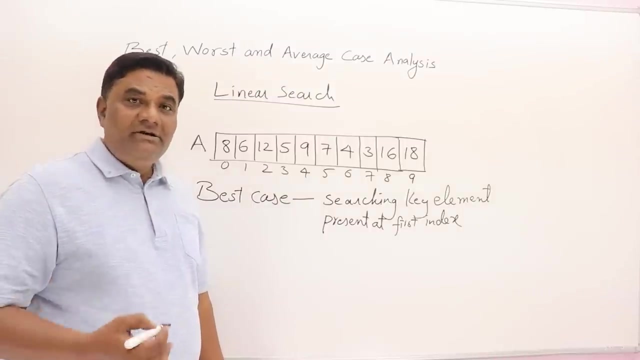 Then what is the existance time of index 8?? The first index is the 我, In this case I. This is best case. Then what is the best case time for the key which is present at index Here in my example? 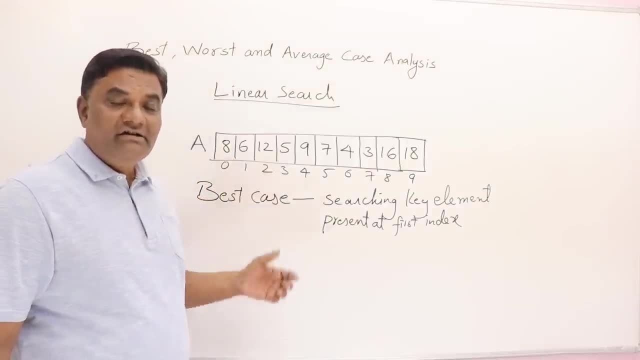 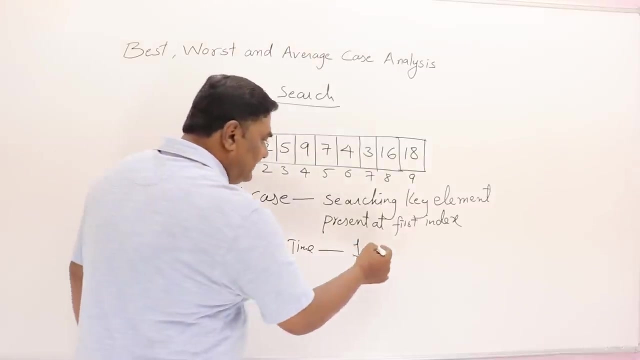 8 is the first key element. if I am searching for 8 then it will take constant time. best case time is constant. I can write it as order of 1, so best case time is for n elements is order of 1. best case time for n elements is order of 1. so here I write: b is 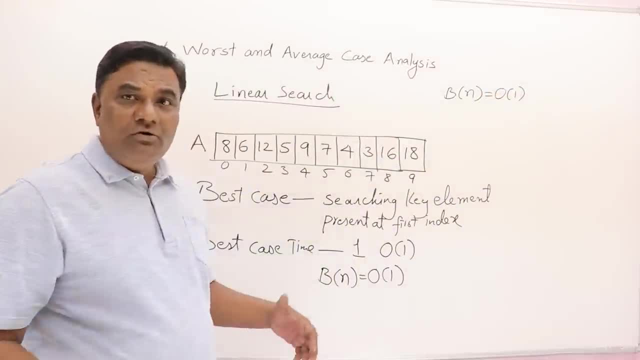 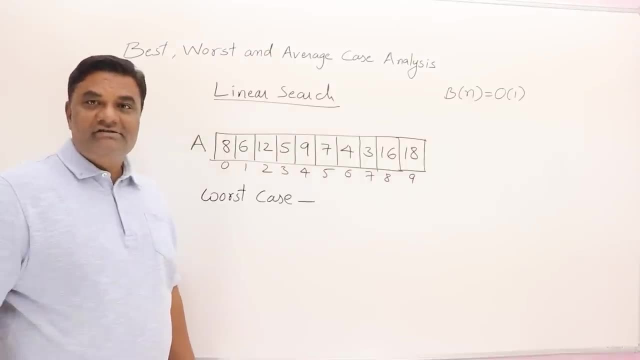 order of 1, now bigger, then omega, which is that will see afterwards. so first I have written that function. now, worst case of an algorithm: linear search algorithm. what is the worst case when the algorithm will take maximum time? if I am a searching forE'. 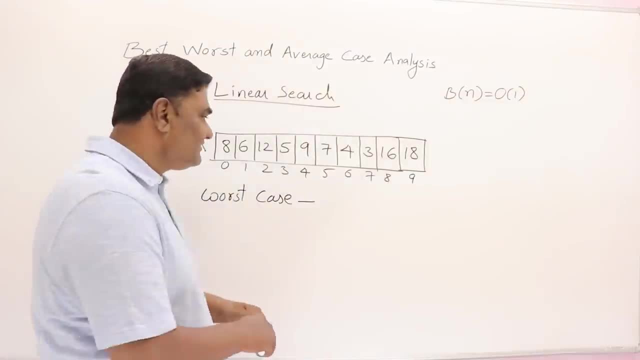 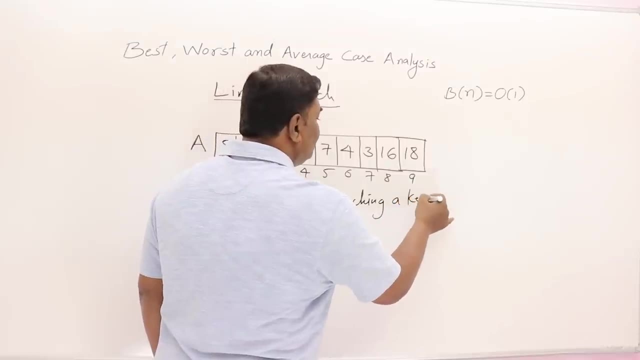 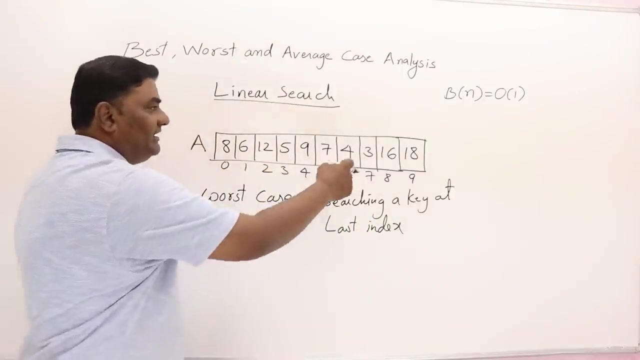 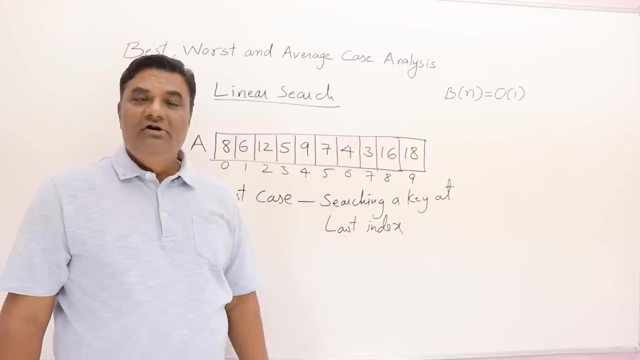 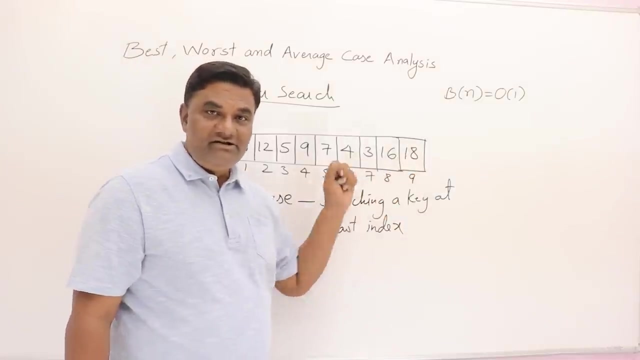 the key which is at the last index. Searching a key at last index. In my example, 18 is the key which is present at last index. So that is the worst case. What's the time taken for searching that key element? So I have to check for all the n elements, then I can reach there. 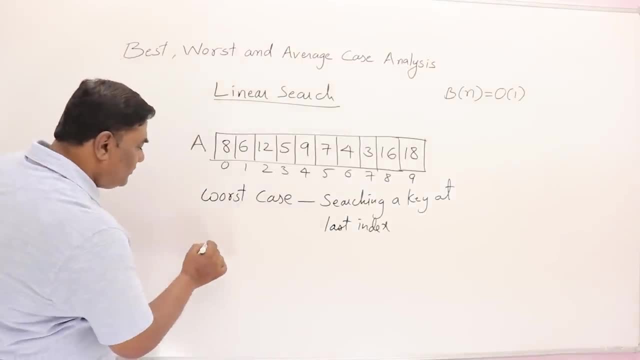 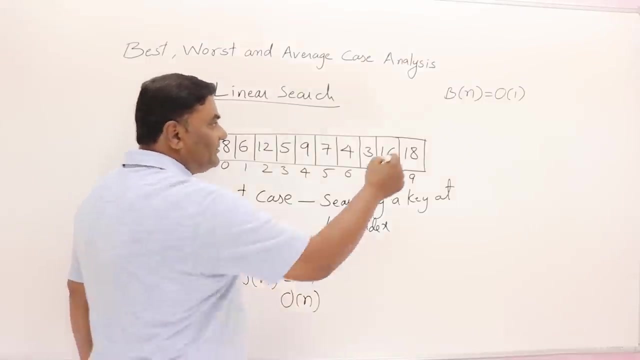 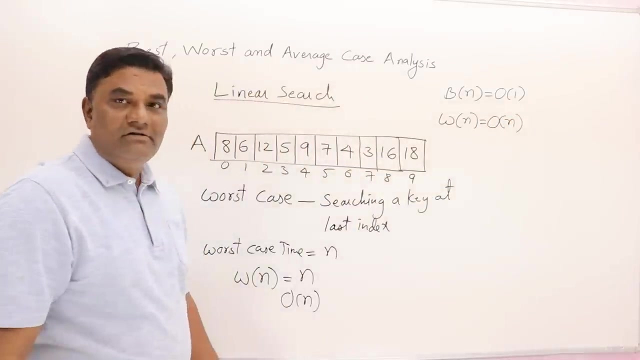 Now what is the time taken in this worst case? Worst case time is n, So worst case for n elements is n and that is order of n. So here I write: worst case for n elements is order of n. So now I have best case as well as worst case times given for linear search, Now average: 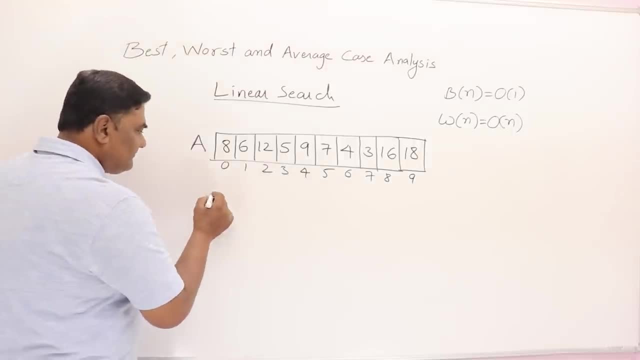 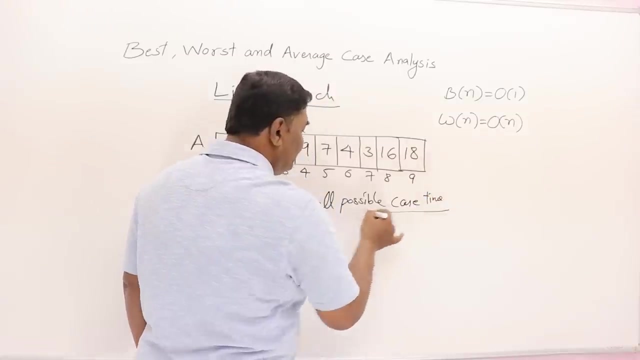 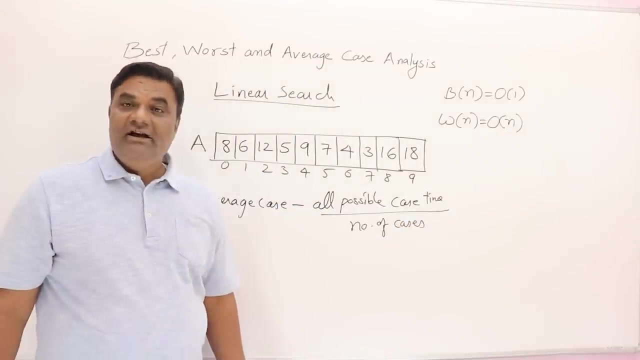 case time. Average case is defined by all possible case time divided by number of cases. So for average case you have to find out all possible cases and the time taken in each possible case and then divided by number of cases. So this type of analysis is very difficult. 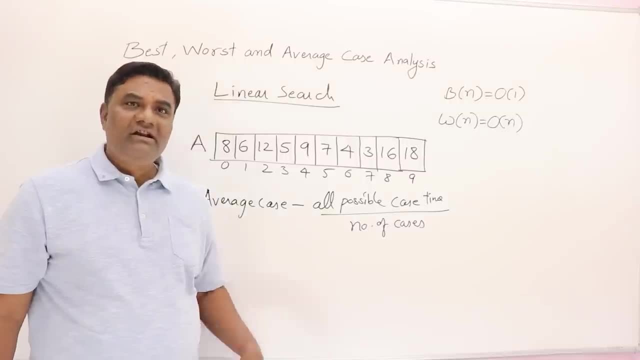 It may not be possible on every algorithm, So rarely we do it, and mostly for average case. the time that we get will be similar to worst case. So that's why we prefer finding worst case time for algorithms, Average case time. Average case analysis may not be possible always. Let us check for linear search. what 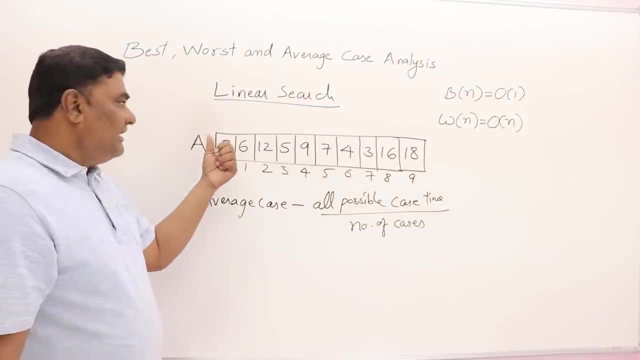 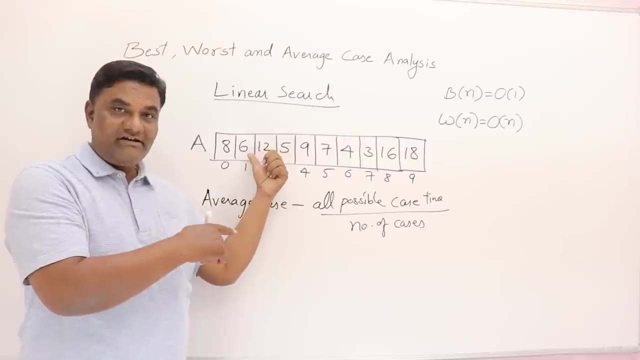 are the cases. So let me tell you this, In case if you are searching for a key present on first index, In case if you are searching for a key present at second index, or in case third index, in case fourth index, in case nth index. So these are all the cases. So 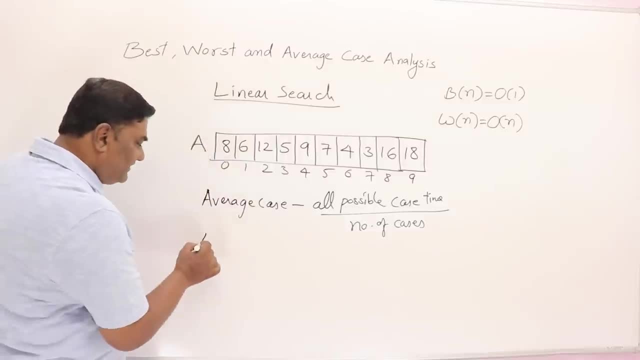 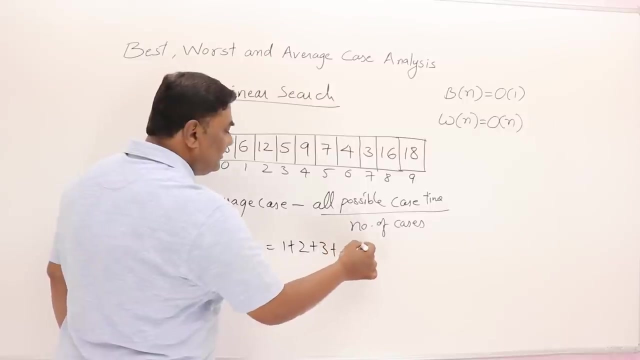 in case, if you are searching for a key present at first index, then average case time is n, For this one it's 1.. If I am searching for a key present at second index, it will take two comparitions and third index, three comparations and so on. And last index is n comparison. 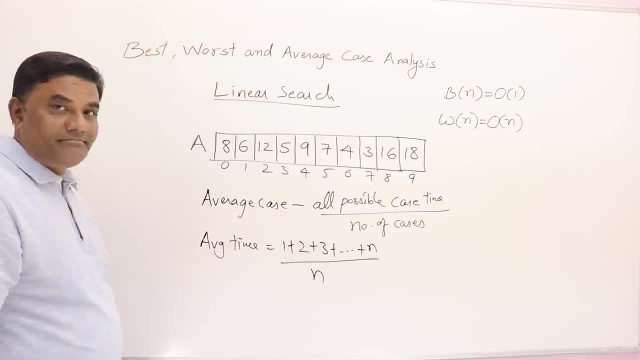 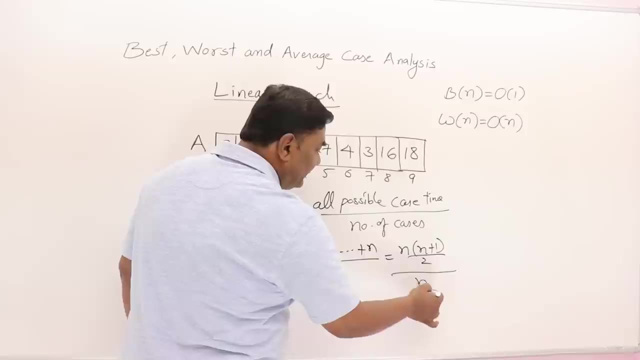 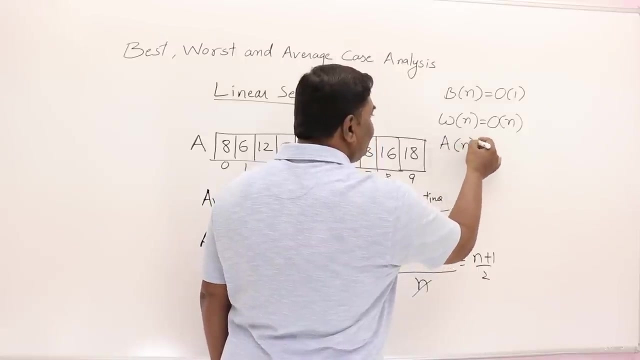 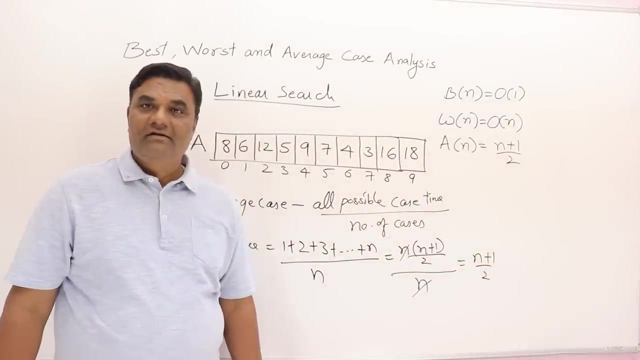 Total cases are there: N. So what does this equal to? This is n × n1 × 2 and divided by n Cancel n. So average case time for n elements is n plus 1 by 2.. All these cases and the time 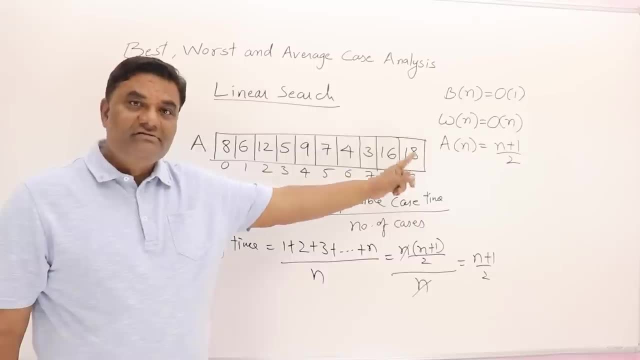 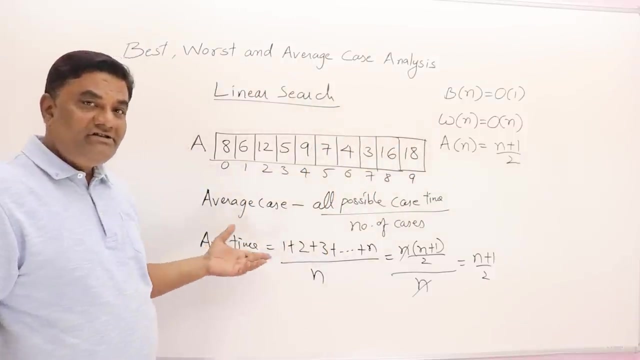 complexities we are finding based on number of comparisons. How many comparisons are required for finding an element Right? so now you have best case and its time and the worst case and its time and the average case. So in average case I consider all possible cases: n elements are there and possible cases. 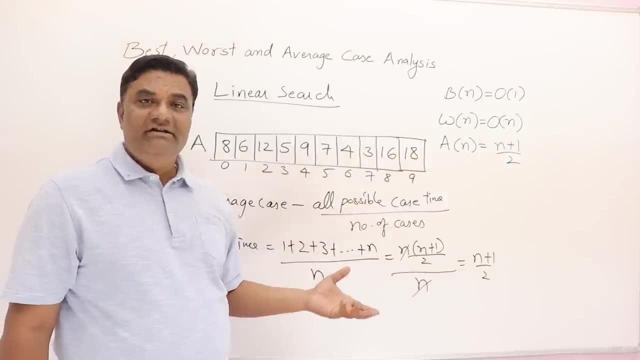 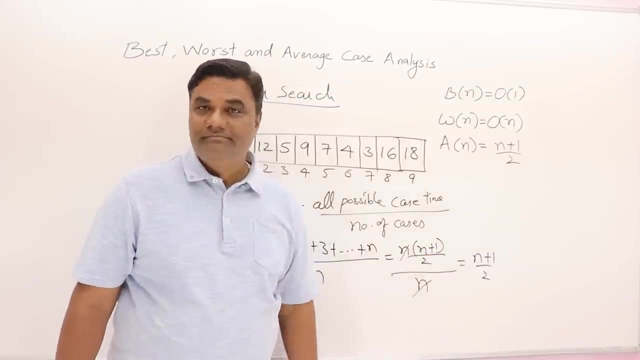 you may be searching for first element or second element or third element, any element. So for each I have taken the time and the number of cases by n, So this is n plus 1 by 2.. Now let us apply asymptotic notations on this one. See I. 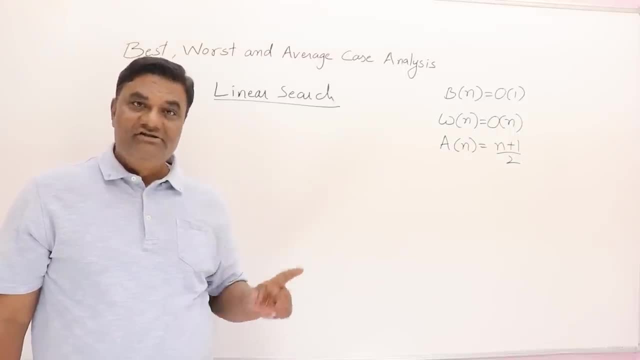 have told you in some video, in one video in asymptotic notation, that cases are no way related to notations. Notations are for the functions. Cases are just the type of analysis done on L'Cordon. Let us see how we can apply notations. See, I have best case time as 1.. Can I write this as best case is big O of n. 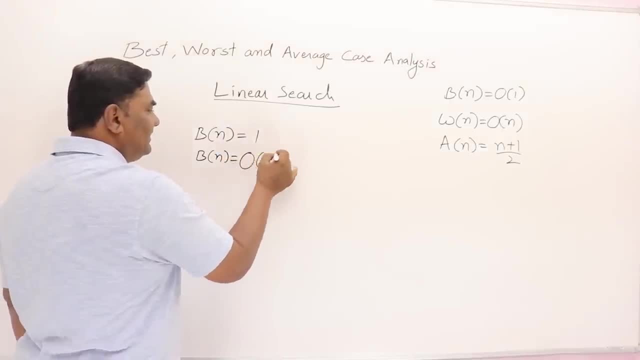 So big O of 1,? yes, I can write big O of 1.. Can I write it as omega 1,? yes, Can I write it as theta 1?? yes, see how. what is the function? function is one constant. so when you have a function constant, 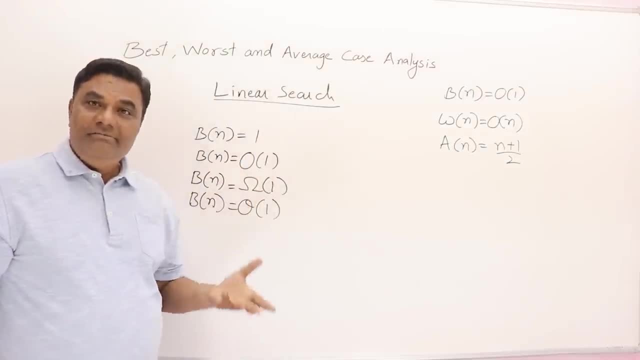 this belongs to constant class. so when it directly belongs to constant class, i can use theta of one, and even i can use upper bound and lower bound also. right this, we have already studied asymptotic notation. so any function greater than equal to comes as upper bound less than equal to comes. 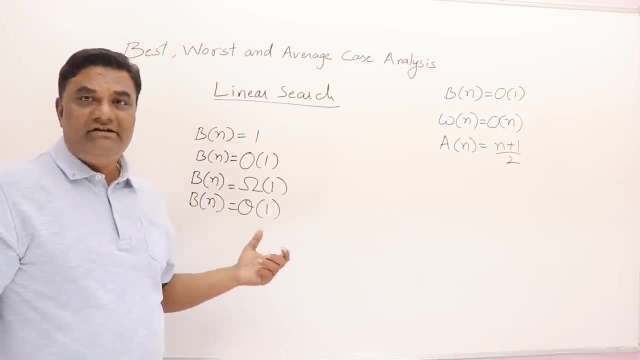 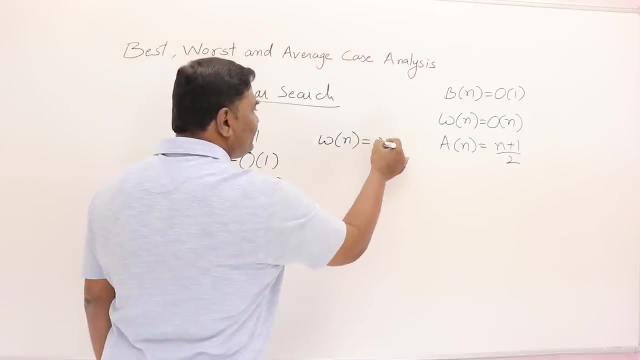 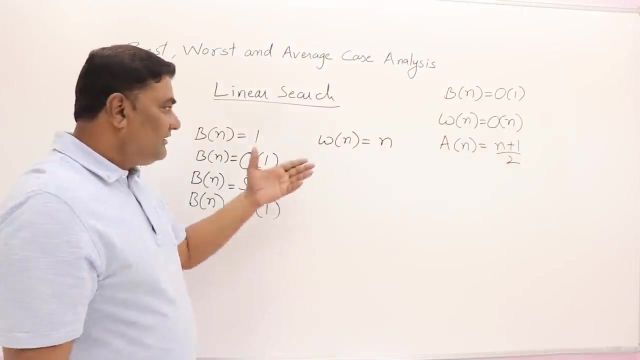 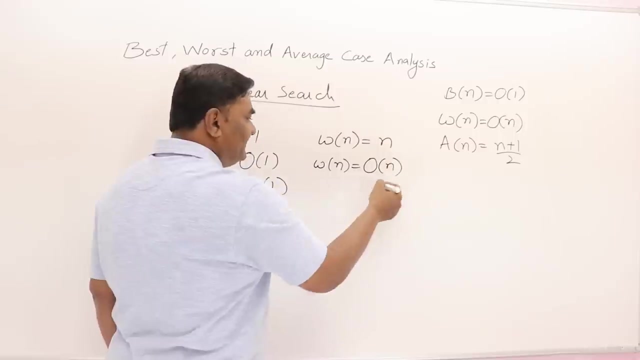 to the lower bound and exactly same function. i just theta. so this is theta. now, worst case, the time is n. this belongs to a class that is linear. function is linear. can i write this as worst case time is is big O of n. yes, worst case of n is omega of n. yes, i can write. 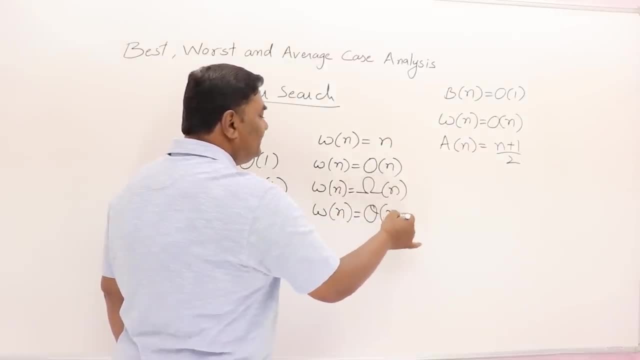 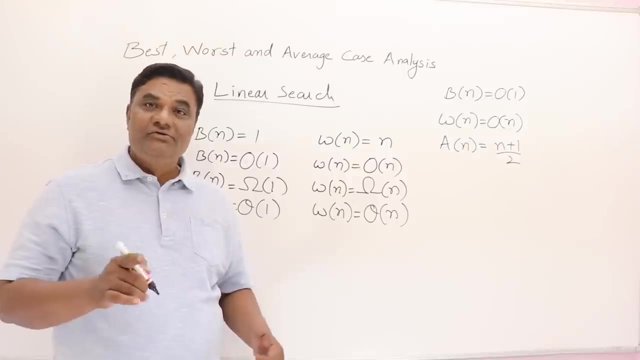 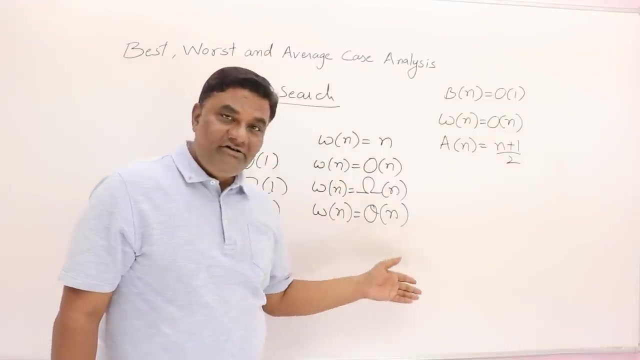 worst case of n is theta of n. yes, I can use any of these notations. there is no fixed notation to show that this is best case. this is worst case. best case can be written using any notation and the worst case can also be written using any. 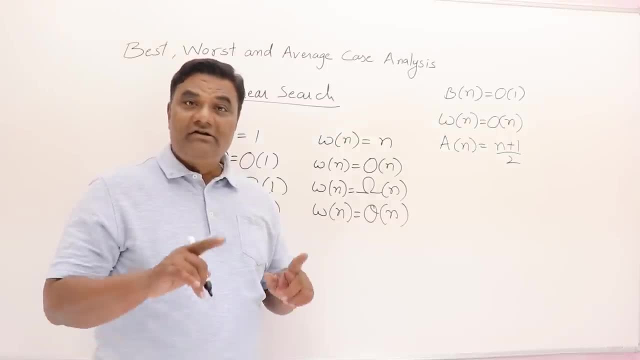 notation right. don't take it wrong: big O is for worst case or Omega is for best case. no, it's wrong. you can use theta also for best case or worst case. you can use big O for any cases and even for average case. I have a function n. 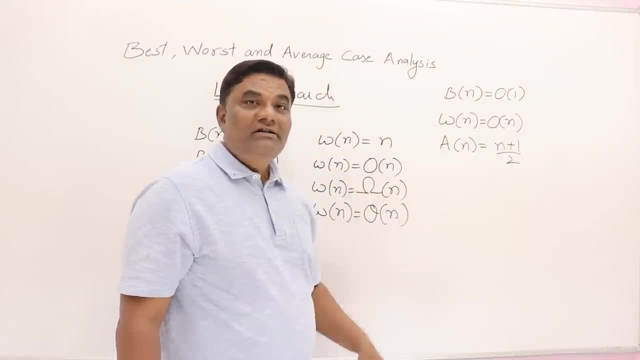 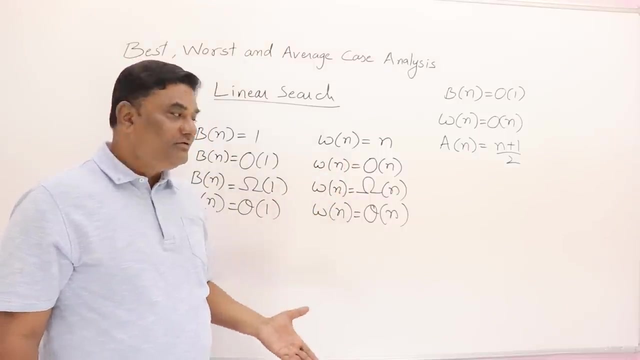 plus 1 by 2. this belongs to which class? it belongs to linear class n, and so even that I can write it as big O, Omega or theta, right? so don't mix up with the cases. that's already I have told you. now I have proved this one right when you 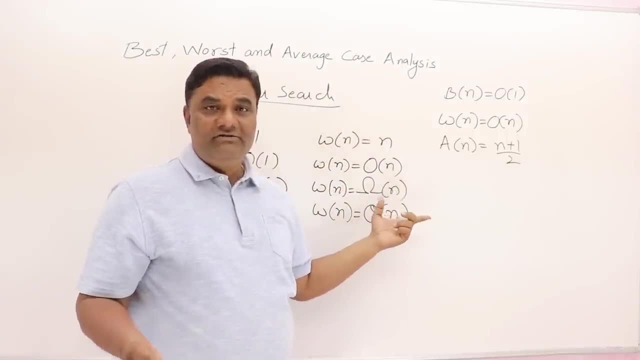 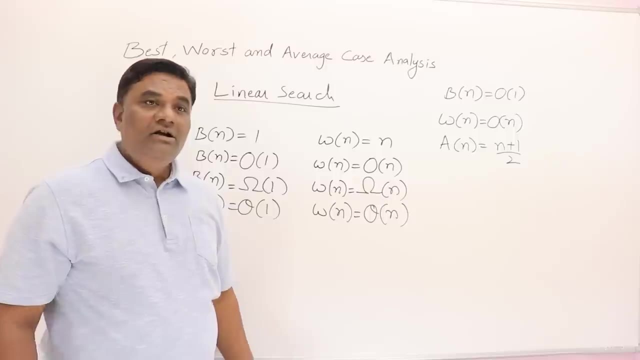 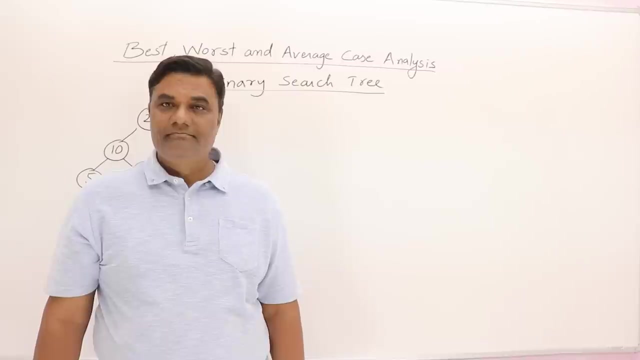 have a function for a function. you can use big O also, Omega also, theta also. all are true, all are correct, right? mostly people confuse that this worst case should be big O. this is upper bound, maximum, upper bound, right, lower bound. so Omega, no, nothing like that. you can use any notation. now. next example is binary. 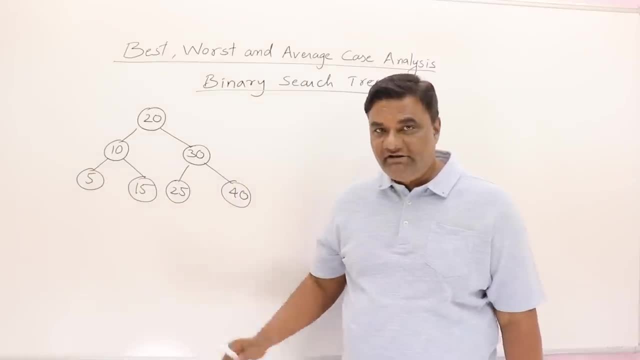 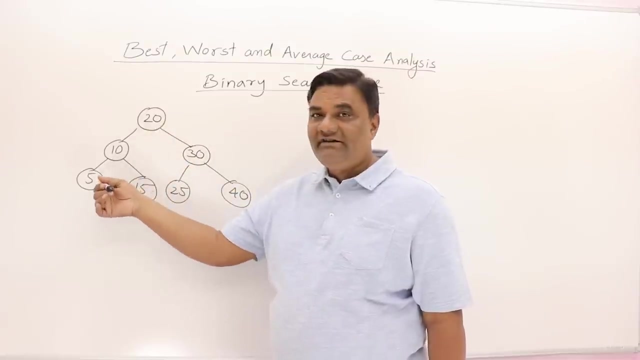 search tree. here I have a binary search tree. I guess I hope that you already know binary search tree. the purpose of binary search tree is useful for searching. the elements are organized such that for every node, all the elements smaller are on the left hand side, all the greater elements on the right hand side. so for 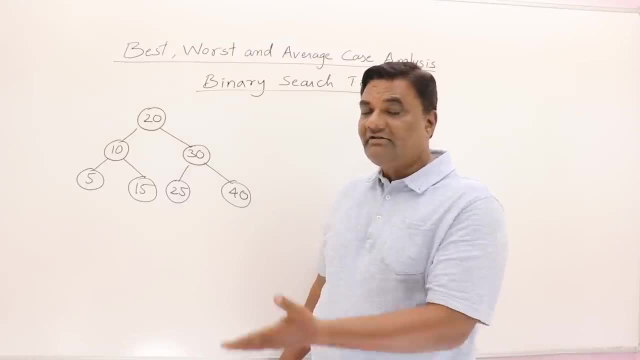 searching. if you are searching for smaller element, we goes on left side, or greater element, we go on right side. suppose I am searching for 15. let me show you the working out. if I'm searching for 15 and start from 20, is it 15? know, 15 is? 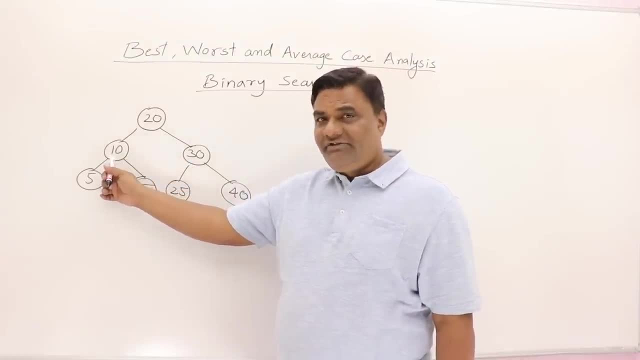 smaller than this one. so we left hand side, is it 15? no, 15 is greater than this one. so go on right hand. yes, 15 is found. so what is the time taken for searching total? how many comparison? I have done only three comparison's. I have done so the time. 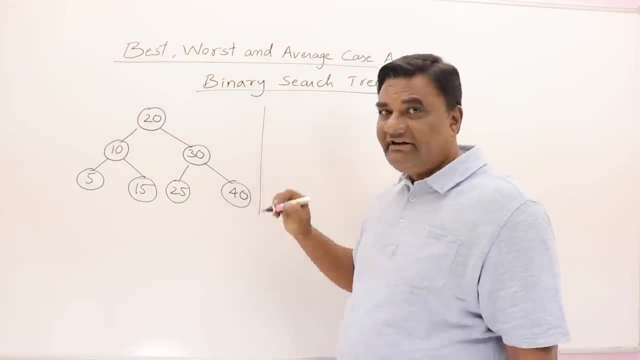 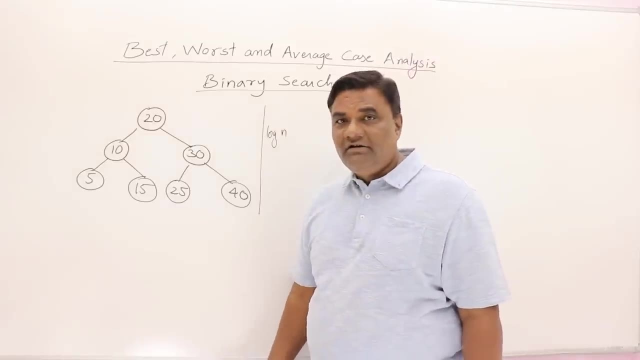 taken is three. so actually that is equal to the height of a tree. height of a tree. so what's the height? we usually call it as log n. log n is the height, So around 7 elements. I have means 8 elements, So log 8 is 3.. So 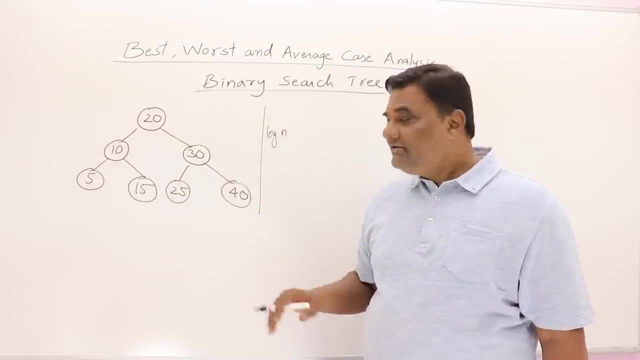 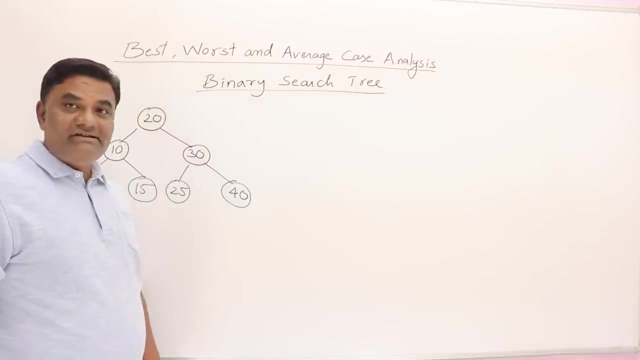 3, comparisons are required. So the height of a tree is log n, So the time taken is log n for 15.. Now let us understand what is best case and what is the best case time. worst case and worst case time. Best case is if I am searching for the element which is present. 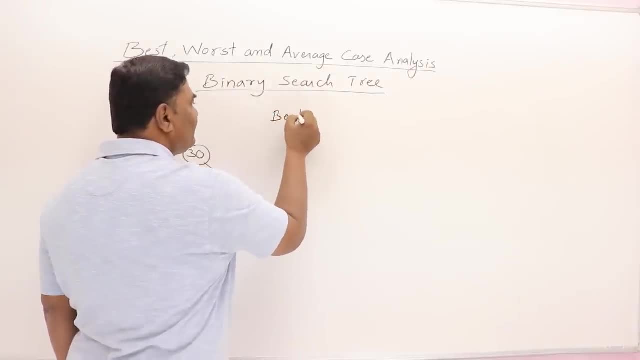 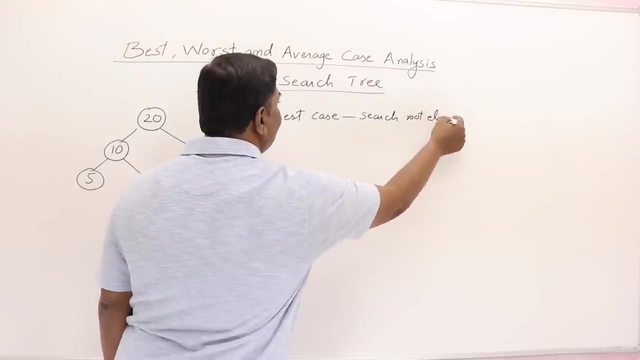 in the root. Best case searching: root element. In short, I am writing means I am searching for the key element which is present in the root. So how much time it will take for searching for that particular element? Just constant time If I am searching for 20, just check. 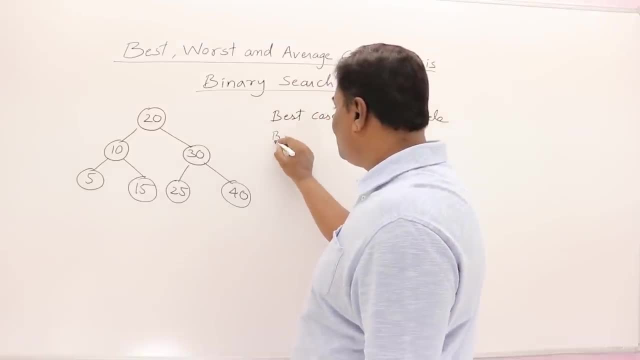 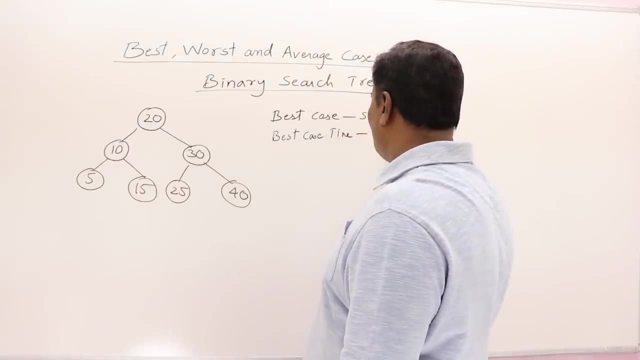 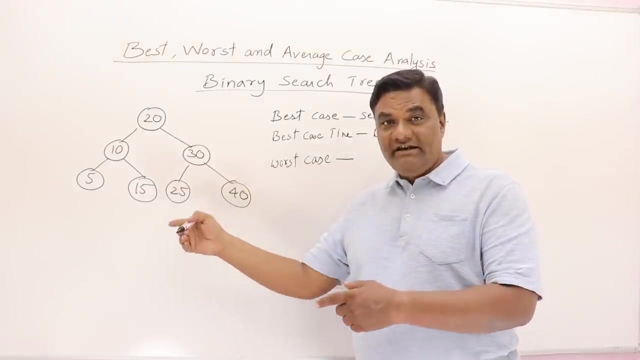 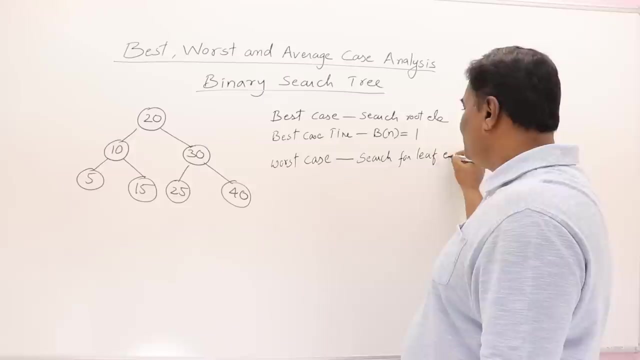 it in the root. Yes, the element is found. So the best case time is best case time is: bn is 1.. bn is 1.. Then what is worst case? Worst case is searching for the element which is present in the leaf, Searching for leaf element. So what are the leaf elements in? 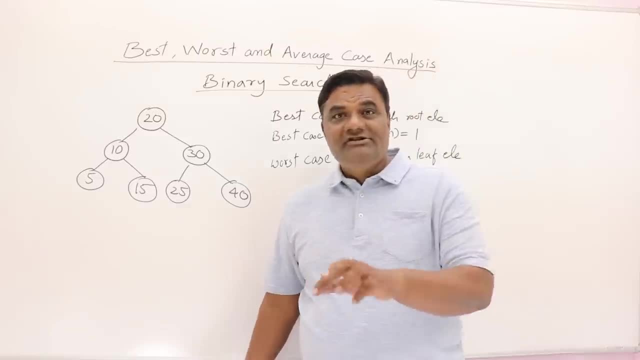 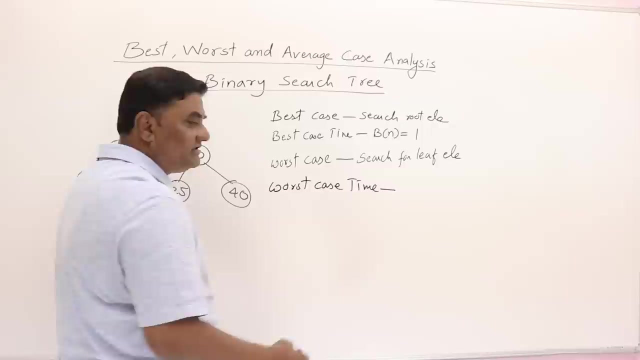 my example: 5, 15, 25 and 40. If I am searching for any one of those elements, then the time will be maximum. That is worst case. So what is worst case time? Worst case time depends on the height of a binary search. 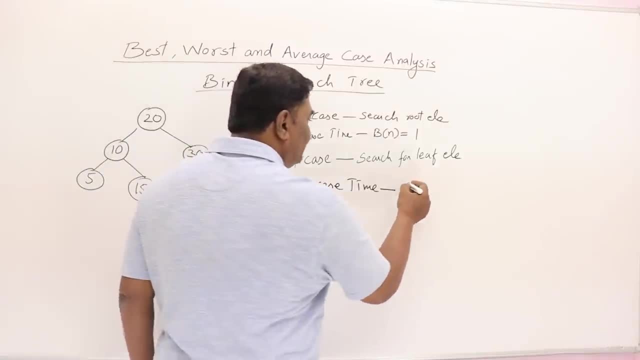 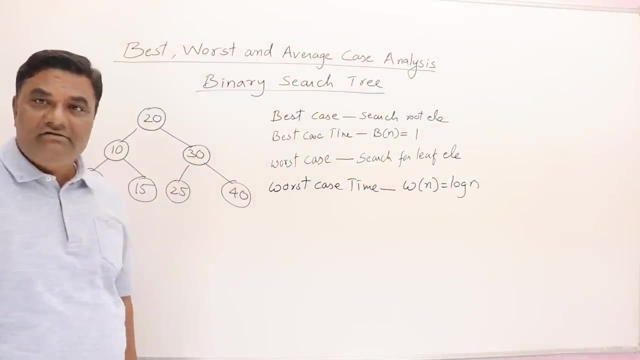 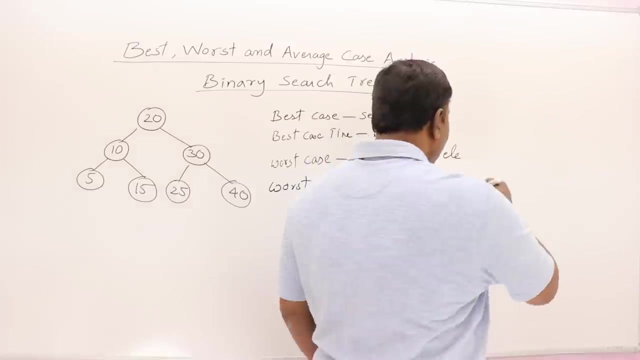 tree. What is the height? Log n. So the worst case is log n. Worst case is log n. So what is the height? 1.. Now this is a binary search tree For the same elements. I can- even I can- have a binary search tree like this: In the root I have 40 and on the left child. 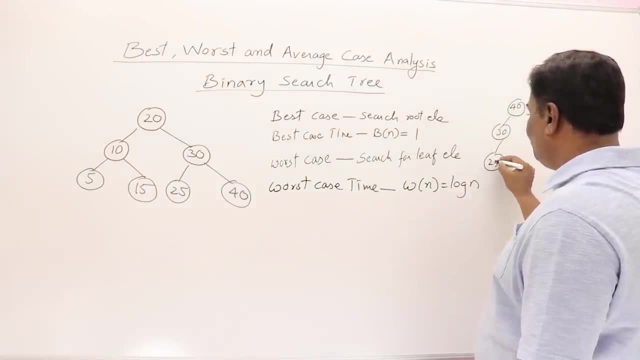 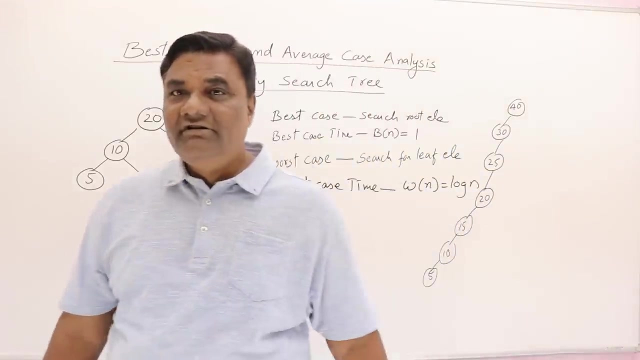 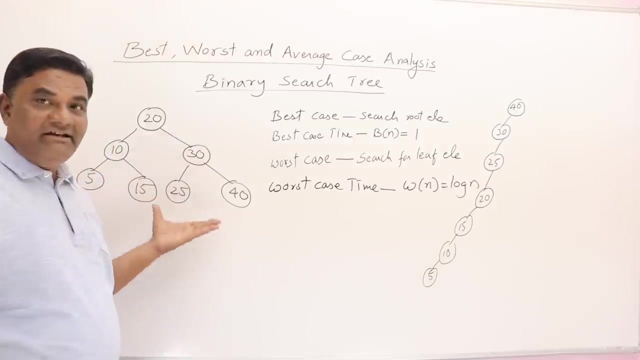 I have 30. On left child 25.. Got it, its left child 20 and its left child is 15 and 10 and 5. this is also a binary search tree. this is a left skewed binary search tree. this is height balanced binary search tree by using: 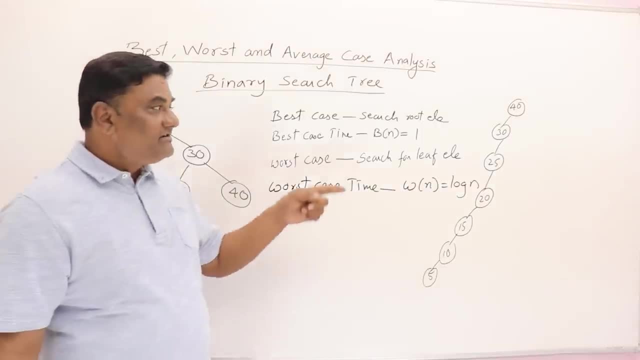 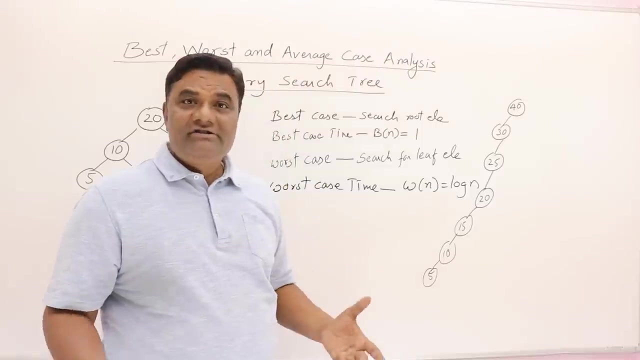 seven elements. this is the minimum height that they can have. this is the maximum height that can I have. now, what is the best case in this binary search tree? best case is same for binary search tree. best case is same: searching for a root- that one. then. what is worst case? searching. 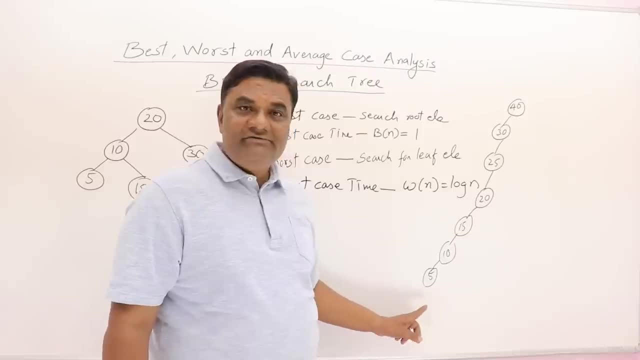 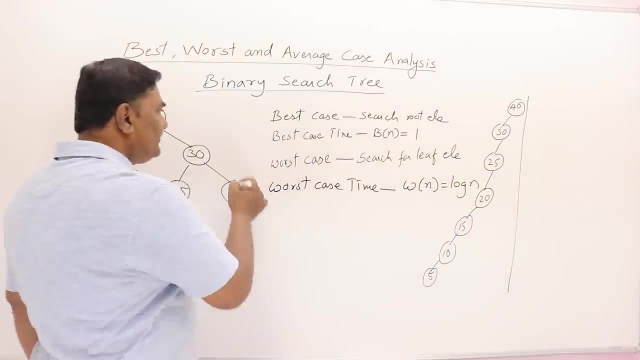 for a leaf. so who is a leaf? only one element. searching for this one is worst case. but what is the time taken depends on the height of a tree, and here also it was dependent on the height of a tree and the height was log n, and here the height is n. 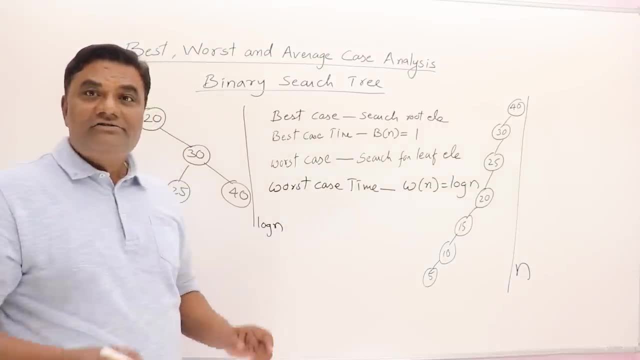 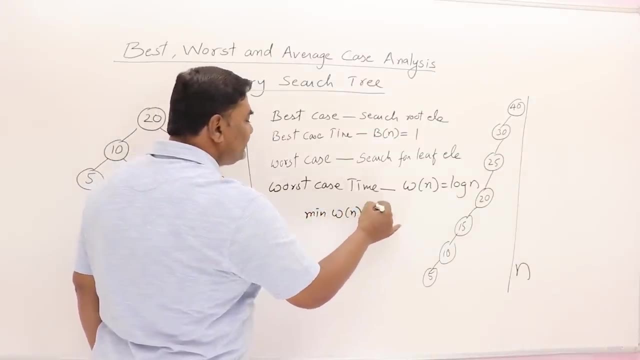 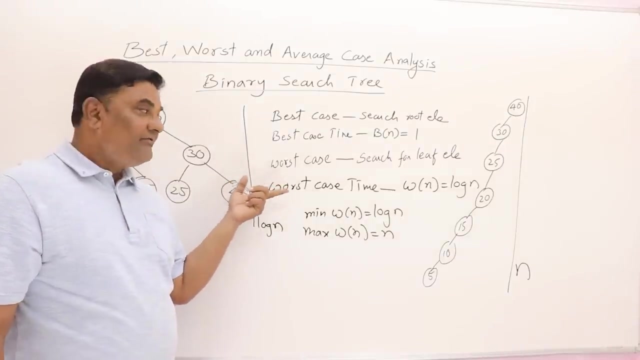 height is n. so it means that in worst case, minimum worst case time is how much log n and maximum worst case time is how much n. so I repeat the point once again. I repeat the point once again. see what's the worst case for binary search tree: searching for an element present in the leaf. 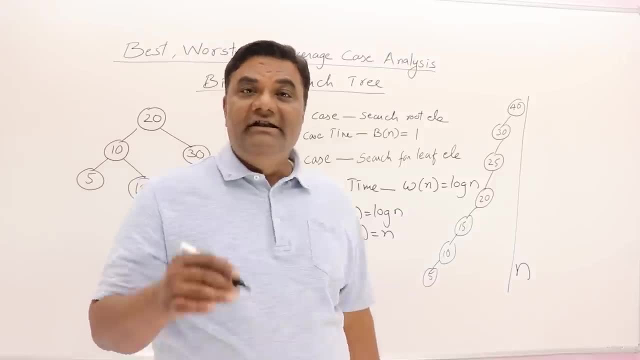 searching for an element present in the leaf that I hope is any less or less than the binary act, onda Byron's set power values. this is my search've, is my ent ovt. and what was, Oh byron's set to zero present in the leaf? that is worst case. then what is the worst case a time it? 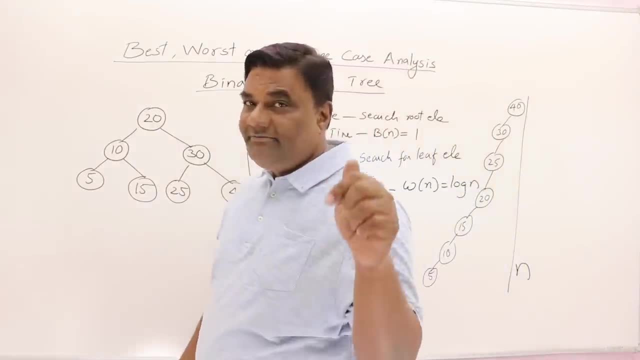 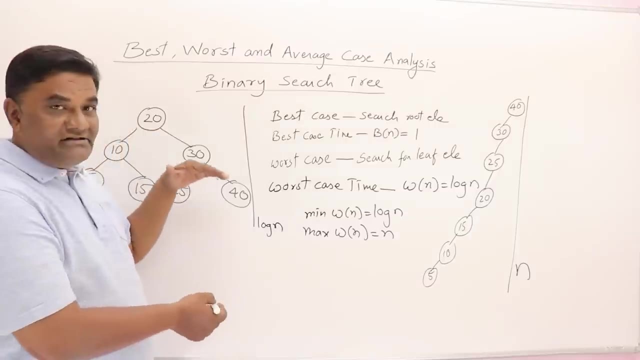 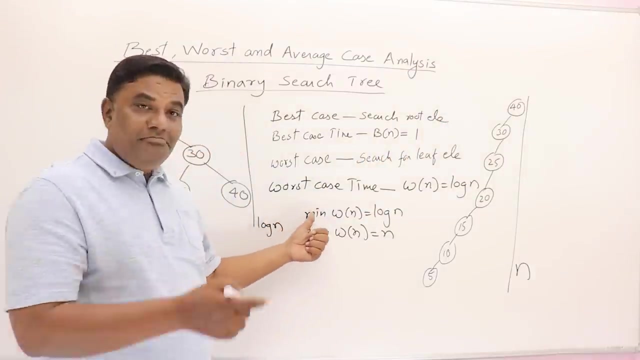 depends on the height of a tree. leaf element will be at the last level. so that depends on the height of a tree. so what could be the height of a binary search tree? the height of a binary search tree can be minimum as log n and maximum as n. so minimum worst case time, maximum worst case time usually.